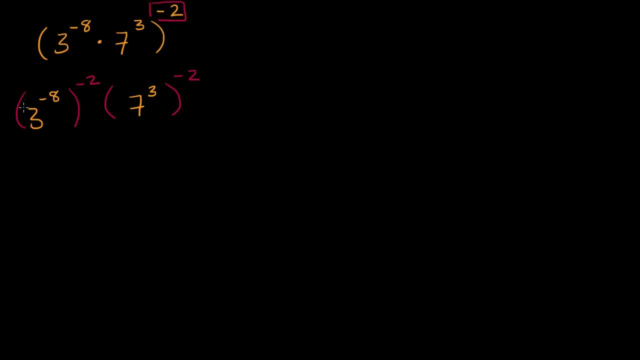 we have the other exponent property that if you're raising to an exponent and then raising that whole thing to another exponent, that you can just multiply the exponents. So this is going to be three to the negative eight times negative two power. Well, negative eight times negative two is positive 16.. 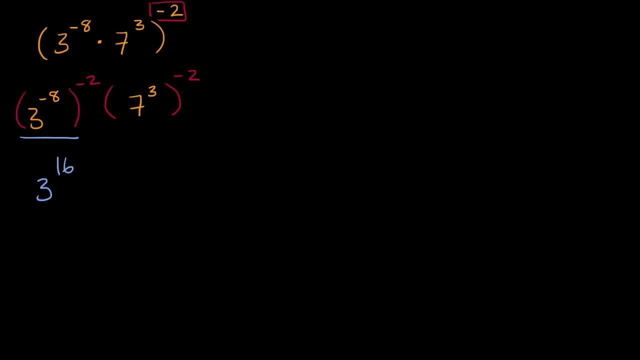 So this is going to be three to the 16th power right over there And then this part right over here: seven to the third, to the negative two. that's going to be seven to the third, seven to the three times negative two. 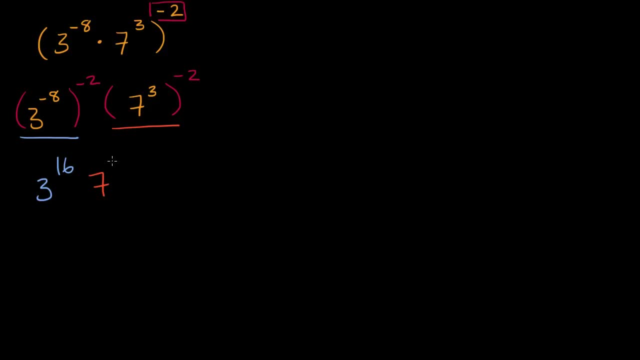 which is seven to the negative sixth power. So that is seven to the negative sixth And this would be about as much as you could simplify it. You could rewrite it different ways. Seven to the negative sixth, the same thing as one over seven to the sixth. 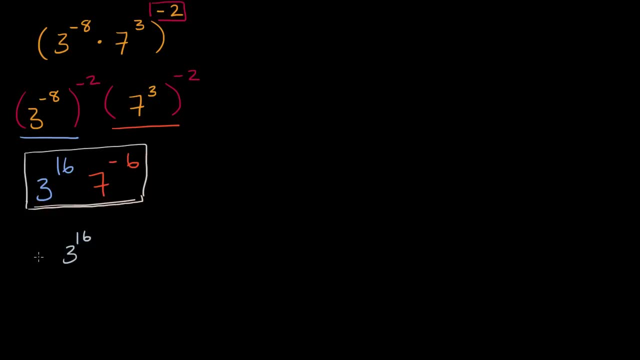 So you could write it like three to the 16th. Let me use that same shade of blue: Three to the 16th over seven to the sixth, But these two are equivalent And there's other ways that you could have tackled this. 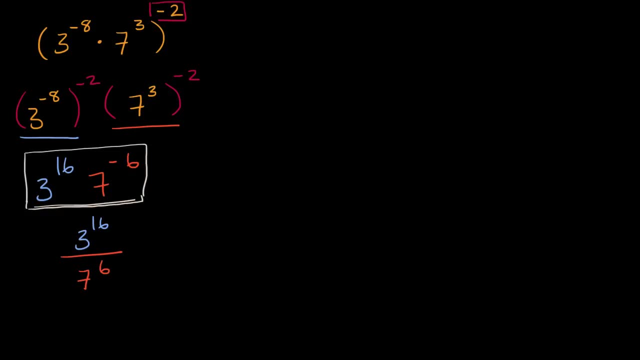 You could have said that this original thing right over here, this is the same thing as three to the negative, eight is the same thing as one over three to the eighth. So you could have said: this is the same thing as seven to the third over three to the eighth. 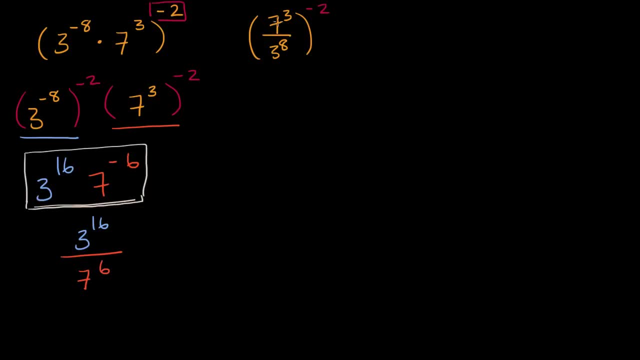 And then you're raising that to the negative two, in which case you would raise this numerator to the negative two and the denominator to the negative two, But you would have gotten to the exact same thing. You would have gotten to the exact same place. 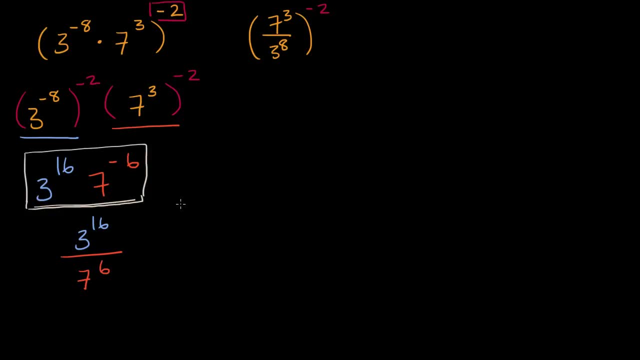 Let's do another one of these. So let's say, let me, so let's say that we have. we have got a to the negative two times eight to the seventh power And we want to raise all of that to the second power. 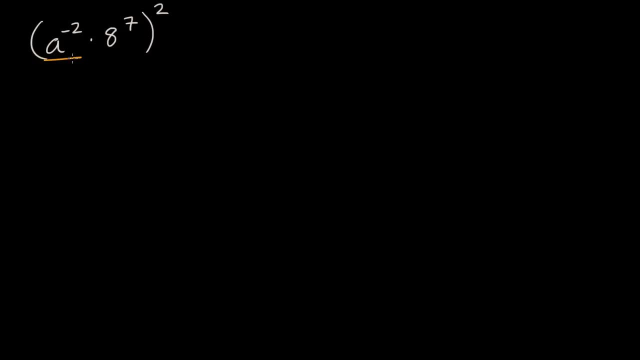 Well, like before, I can raise each of these things to the second power. So this is the same thing as a to the negative two to the second power. times this thing to the second power, Eight to the seventh to the second power, And then here, negative two times two is negative four. 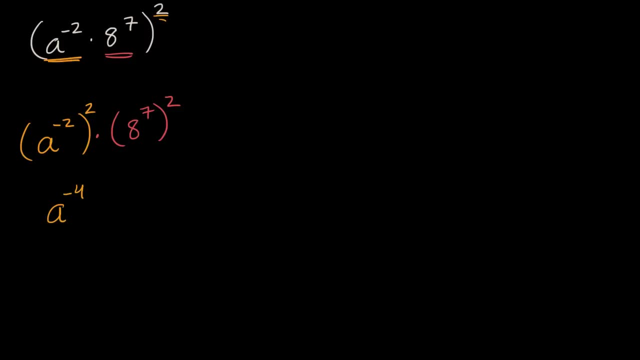 So that's a to the negative. four times eight to the seven times two is 14.. Eight to the 14th power. In other videos we go into more depth about why this should hopefully make intuitive sense. here you have eight to the seventh times eight to the seventh. 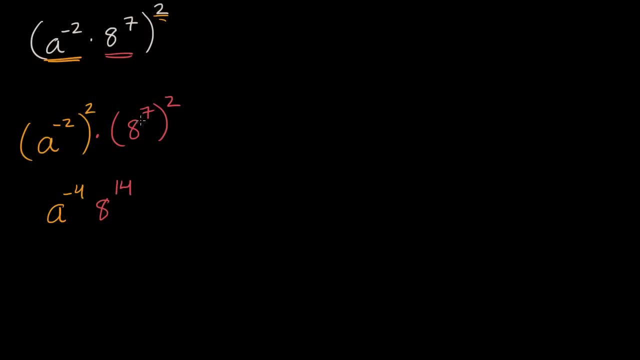 Well, you would then add the two exponents and you would get to eight to the 14th. So however many times you have eight to the seventh, you would just keep adding the exponents or you would multiply by seven that many times. Hopefully that didn't sound too confusing. 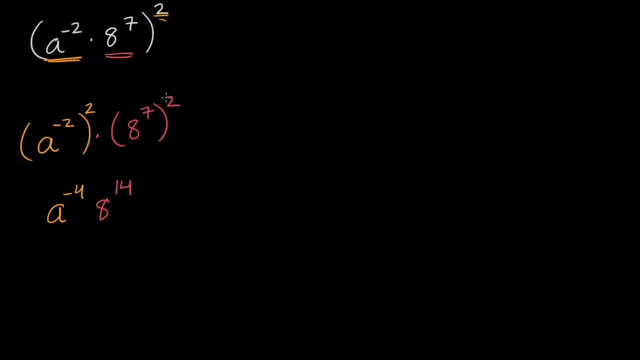 But the general idea is, if you raise something to an exponent and then another exponent, you can multiply those exponents. Let's do one more example where we are dealing with quotients, Which that first example could have even been perceived as. So let's say we have. 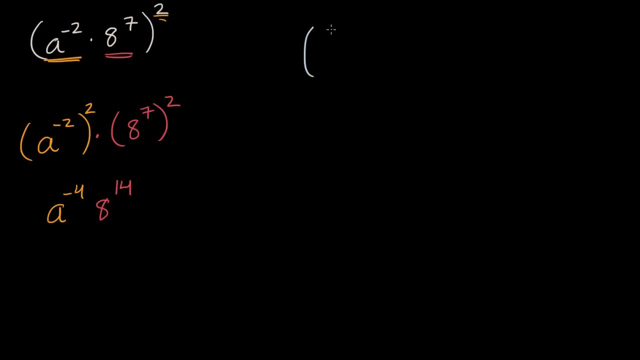 let's say we have two to the negative 10 divided by four squared, And we're gonna raise all of that to the seventh power. Well, this is equivalent to two to the negative 10 raised to the seventh power over four squared raised to the seventh power. 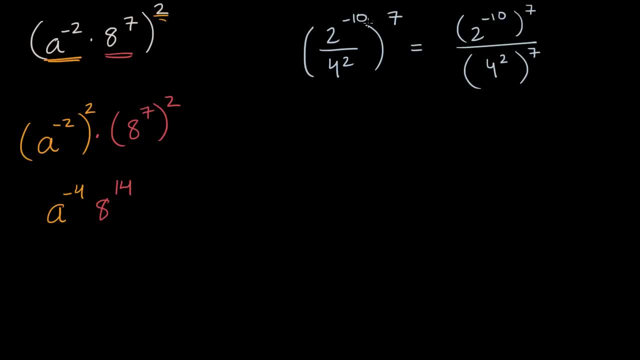 So if you have the difference of two things and you're raising it to some power, that's the same thing as the numerator raised to the power. That's the same thing as the numerator raised to the power. That's the same thing as the numerator raised to that power. 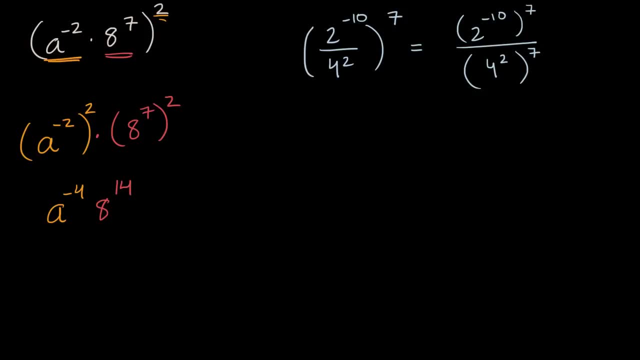 divided by the denominator raised to that power. Well, what's our numerator going to be? Well, we've done this drill before. It'd be two to the negative, 10 times seventh power. So this would be equal to two to the negative, 70th power. 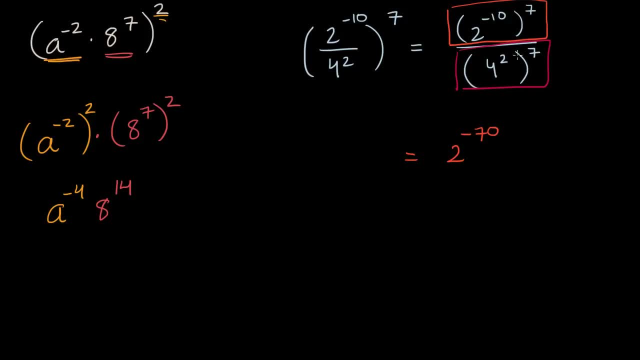 And then in the denominator four to the second power, then that raised to the seventh power. well, two times seven is 14.. So that's going to be four to the 17th, four to the 17th power. Now we actually could think about simplifying this even more. 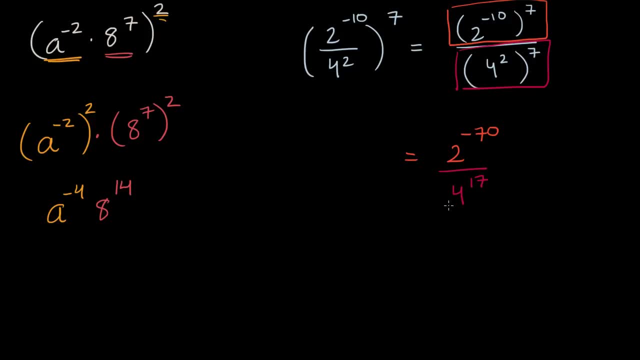 Now we actually could think about simplifying this even more. There's multiple ways that you could rewrite this, But one thing you could do is say: hey look, four is a power of two. So you could rewrite this as this is equal to two, to the negative 70th power. 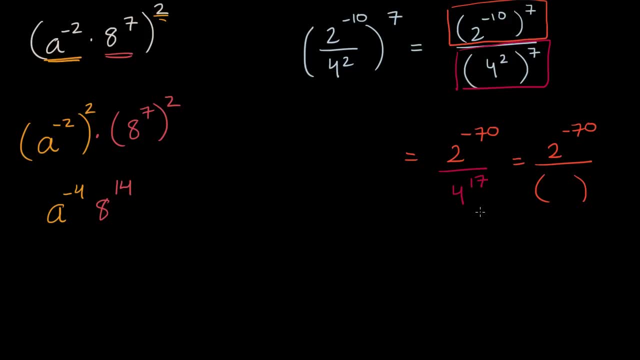 over instead of writing four. instead of writing four to the 17th power. why did I write 17th power? It should be four to the 14th power. Let me correct that. Instead of writing four to the 14th power. 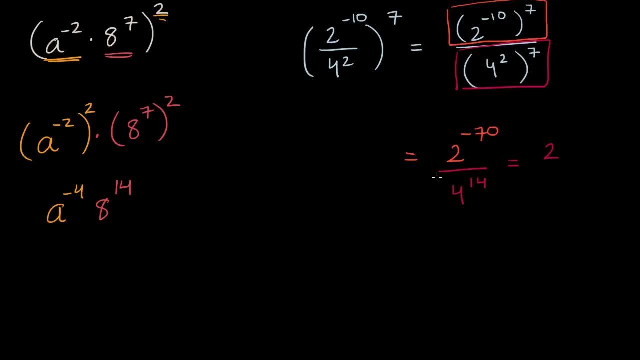 I instead could write: so this is two. let me get the colors right. This is two to the negative 70th, over over. instead of writing four, I could write two squared to the 14th. power Four is the same thing as two squared. 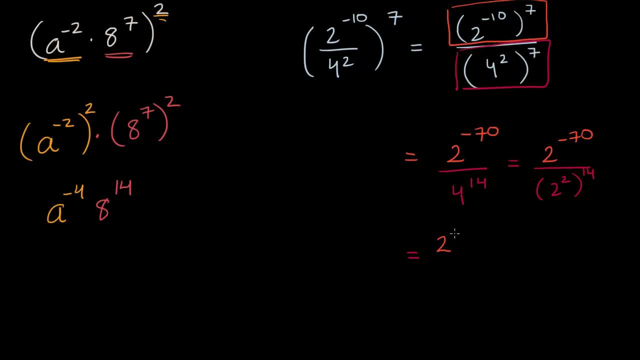 And so now I can rewrite this whole thing as: two to the negative 70th power, over, over, over well, two to the second, and then that to the 14th. well, that's two to the 28th power, Two to the 28th power. 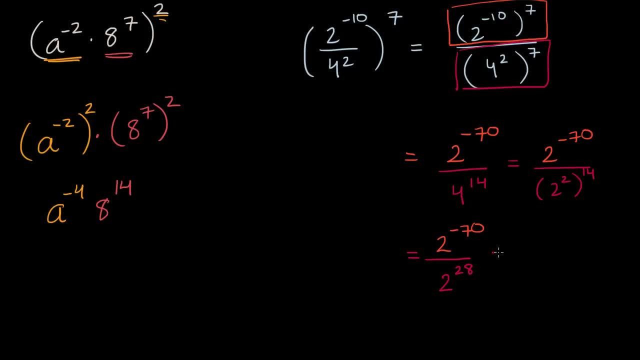 And so can I simplify this even more. Well, this is going to be equal to two. to the I can, just if I'm taking a quotient with the same base, I can subtract the exponent, So it's gonna be negative 70.. 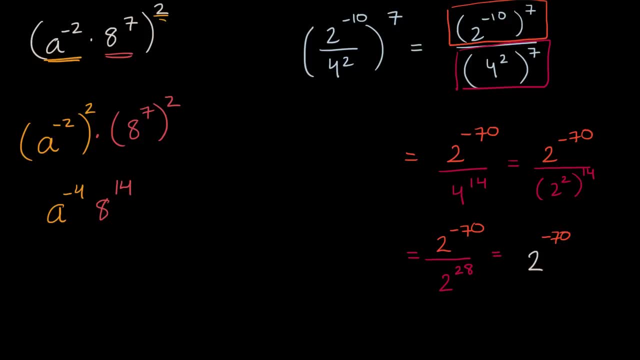 It's going to be negative: 70 minus 28th power Minus 28.. And so this is going to simplify Two to the negative 98th power, And that's another way of viewing the same expression. 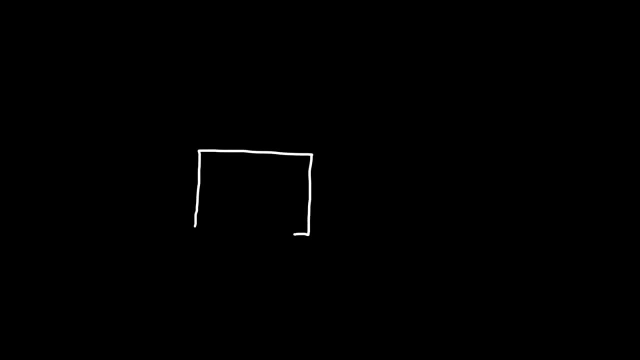 Now in this lesson we're going to calculate the surface area of a cube. Now what's the formula for that? How can we calculate the surface area of a cube? So all sides of a cube are the same. Now let's say, if you want to calculate the area of one of the six faces? 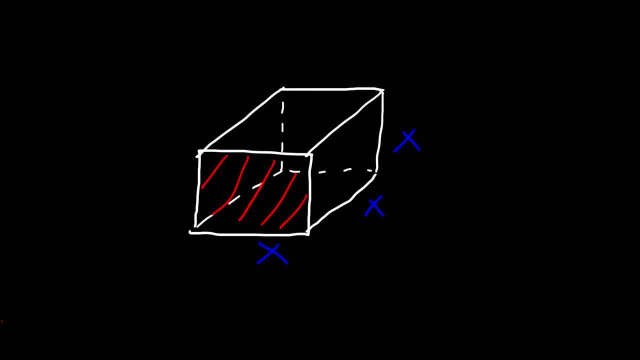 Let's say the area of this face. It's going to be the length times the width. Now both the length and the width is equal to x. So if the area of one face is x times x or x squared, and each face is the same,